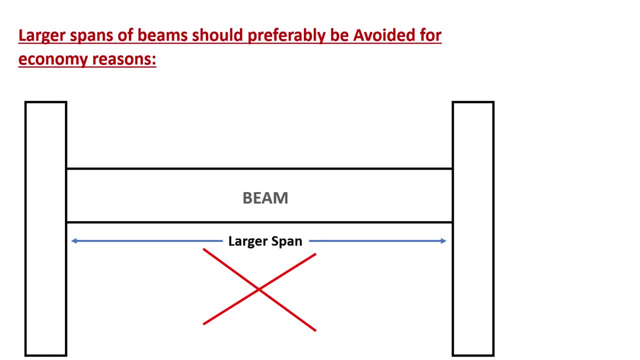 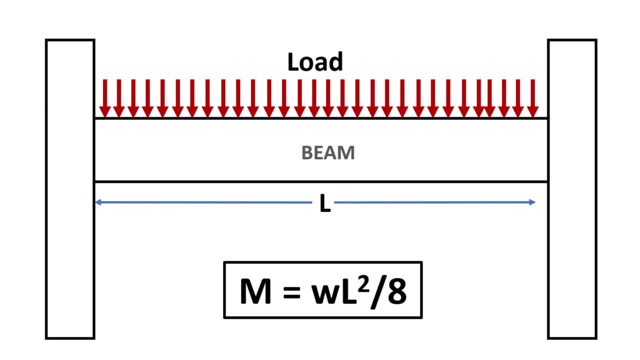 increased, thus increasing its self-weight and total load, because the moment governing the beam design is directly proportional to the square of the span and load, as evident from the bending moment equation. Therefore, a larger span for the beam leads to a notable increase in size, is amenable to the speed to which the beam 75 G is under relocation. However, 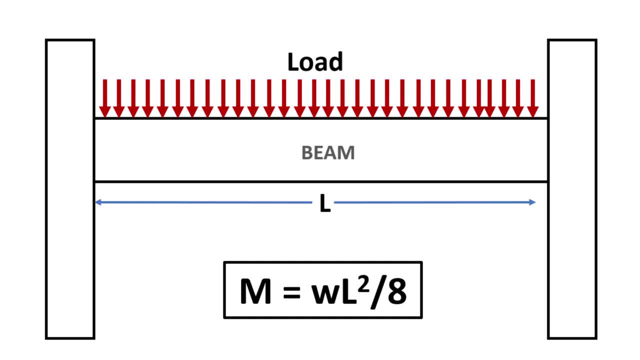 in the size, that's, the depth of the beam. When it comes to columns, the impact due to increase in length on the total load and column size is negligible as long as the column is short. As a result, columns are generally more cost-effective. 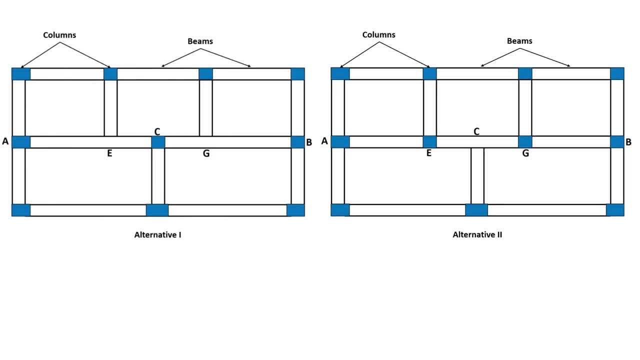 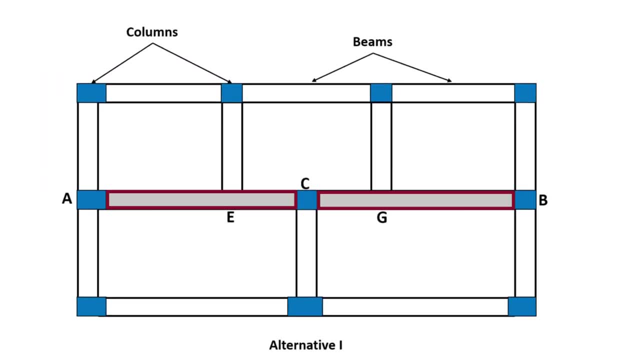 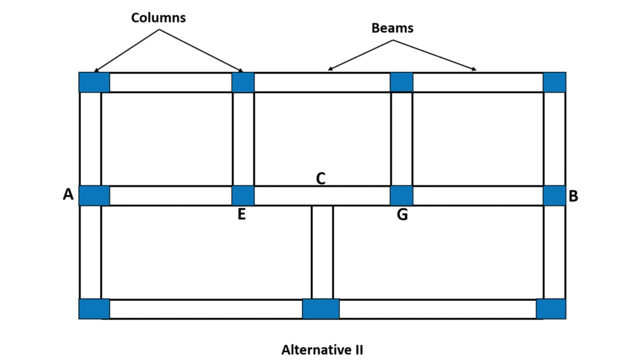 compared to beams in terms of unit cost. Let's consider the structural layout as depicted in this picture, which presents two alternatives. To create a 2-span continuous beam for AB, a single column can be placed at C. Alternatively, two columns can be installed. 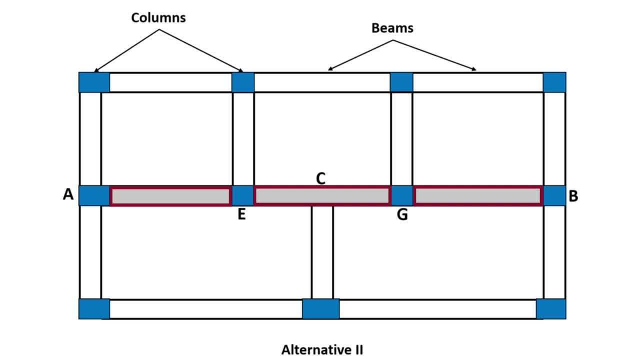 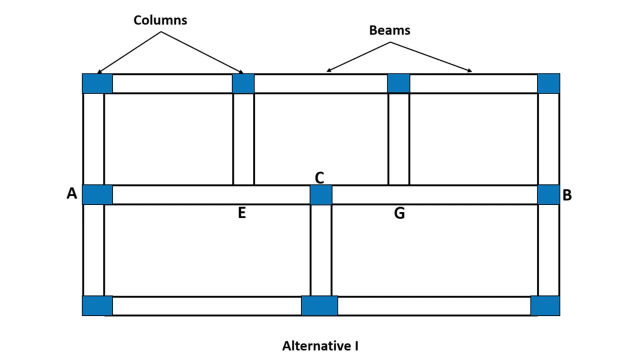 at E and G to form a 3-span continuous beam for AB In case 1, spans AC and CB will be larger and the beam will have to carry two point loads, one at E and the other at G, transferred from secondary beams. 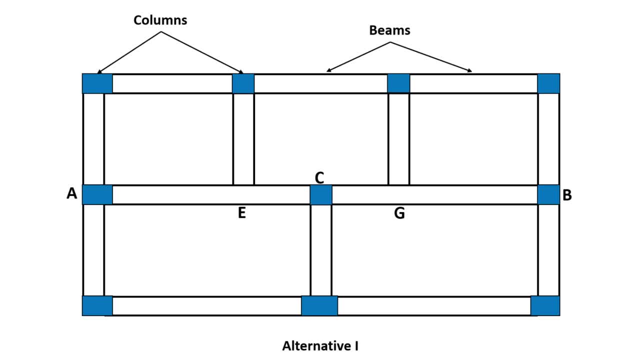 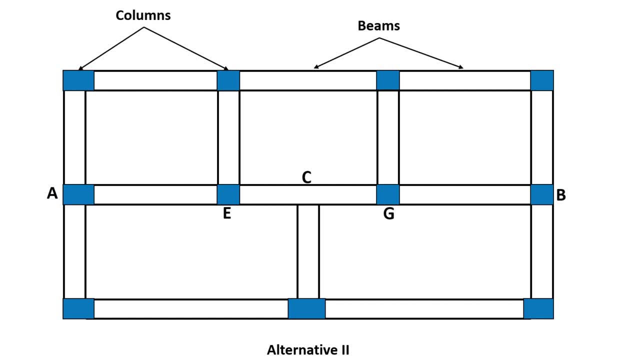 This will require a heavier section for the beam. On the other hand, in case 2, with two columns provided at E and G, the beam becomes a 3-span continuous beam. The length of the beam is reduced and it only needs to carry one point load. 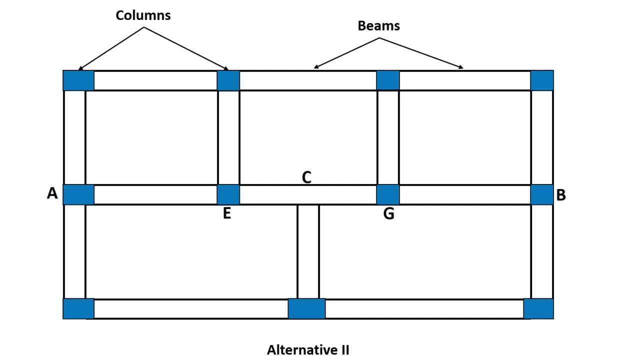 at C, which is located on the central span. This further reduces the bending moments in the outer spans AE and GB without a significant increase in design moment in portion EG, resulting in a considerable reduction in the cost of the beam. Hence the increase in cost due to. 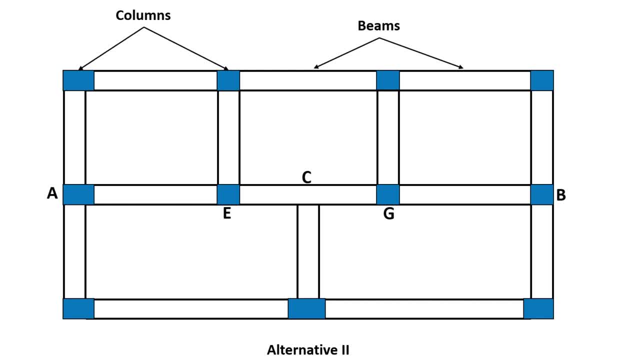 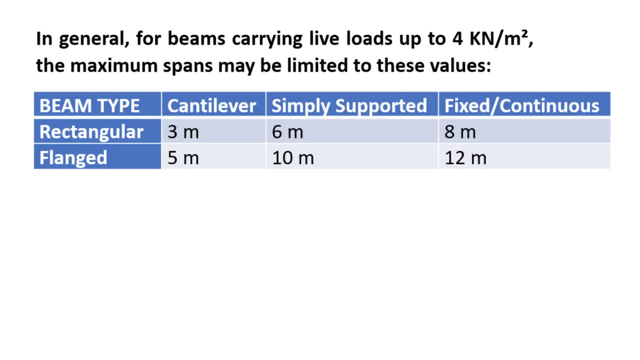 provision of two columns at E and G compared to the single column at C is likely to be relatively less than the increase in the cost of the beam when providing a single column at E. Therefore, second alternative is expected to be more cost-effective In general for beams carrying 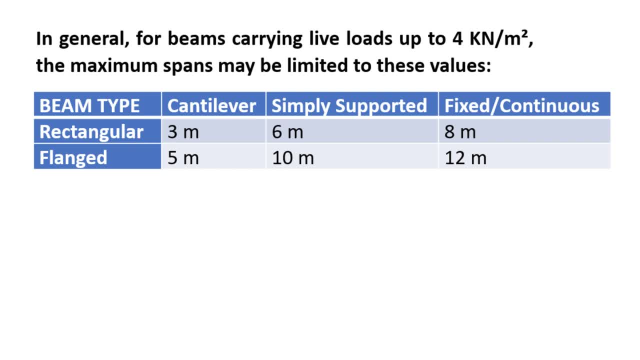 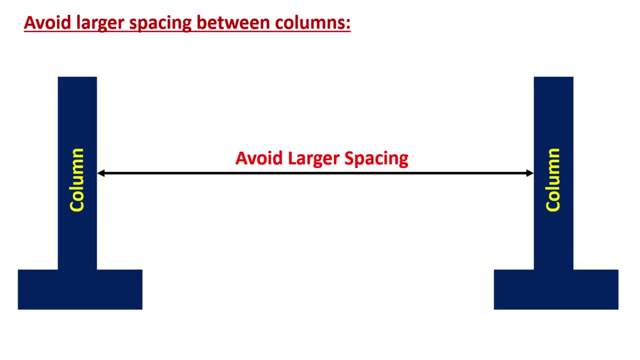 live loads up to 4 kN per m2, the maximum spans may be limited to these values. It's also important to avoid larger spacing between columns. Larger spacing between columns not only results in longer spans for beams, but also increases the load.